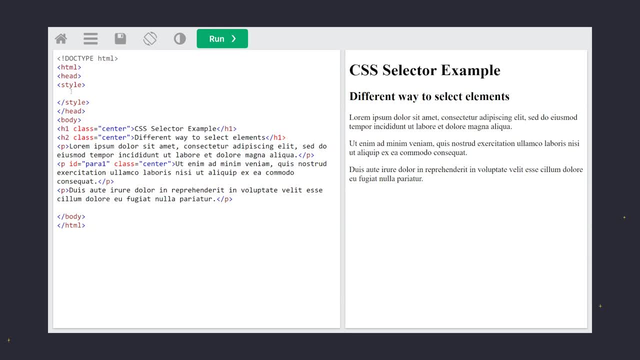 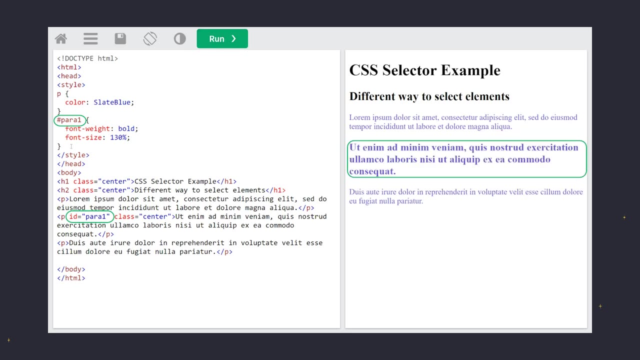 watch as we target the p elements simply by using tag name. We use an element selector, meaning that we use tag or element name. Next, we focus on an element with the ID para1, using the ID selector, which is marked by a hashtag symbol. The ID of an element is unique, so the ID selector is.